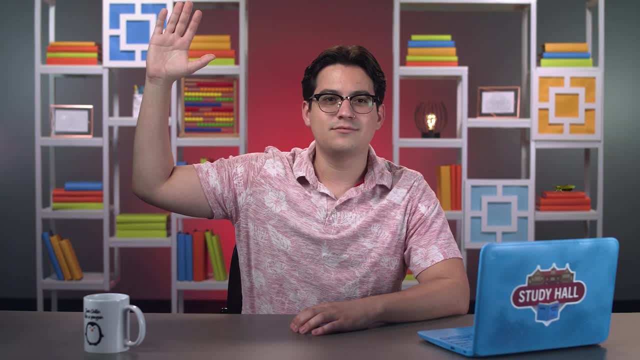 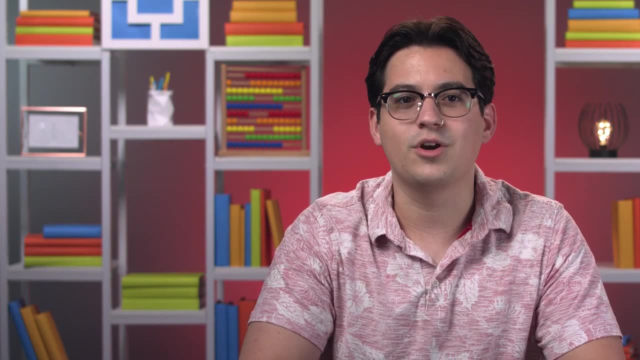 these decisions we have to make. Just me, For instance, a part-time introvert, may need to consider how likely it is they'll have to deal with a crowd before going to any store in the mall, Like some stores might be packed because of a sale or there are stores that 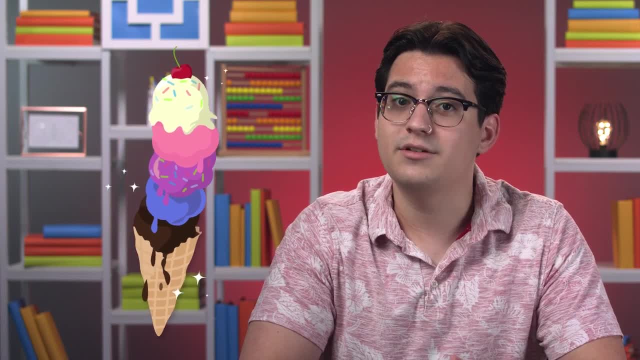 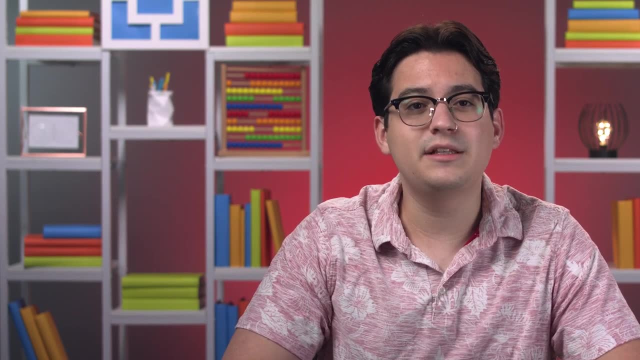 are more popular during certain seasons, like ice cream places in the summer. So which one should they go to, or could they brave both? And if trusting our gut feeling isn't enough, figuring out the probabilities of people being at their favorite store might be a well-calculated 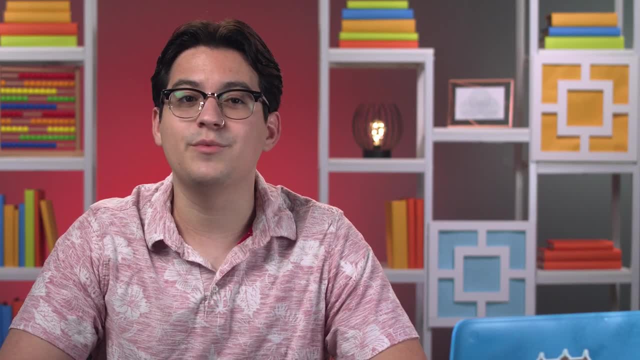 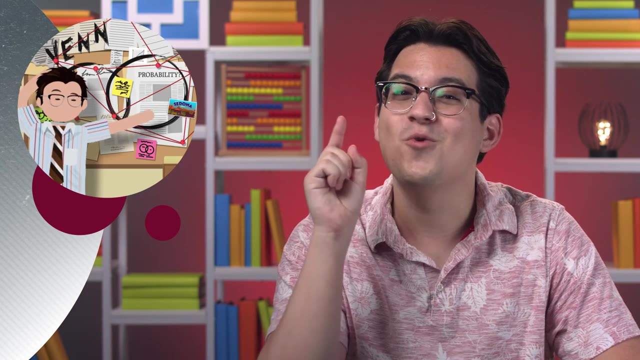 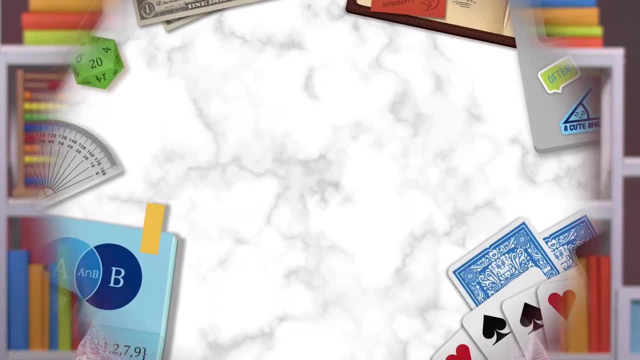 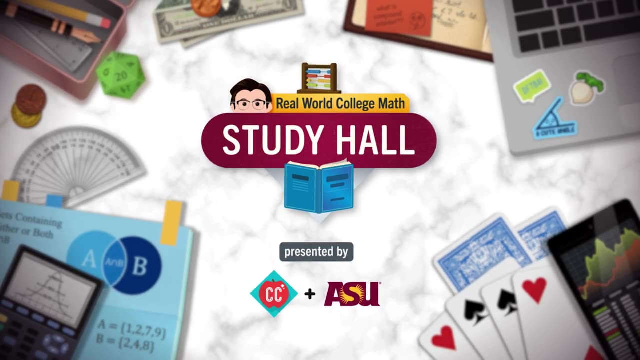 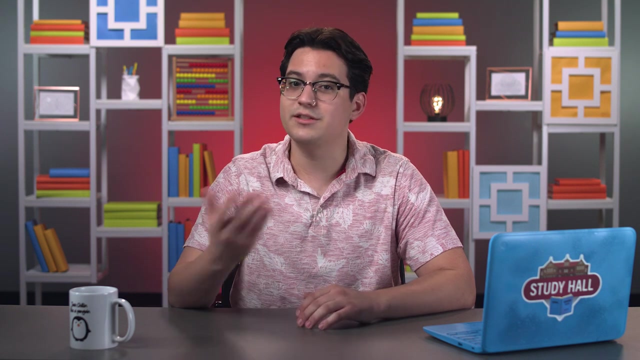 I'm Jason Guglielmo and this is Study Hall Real-World College Math. Last episode we started talking about probability, which is a way of describing the chance something will happen with a number between 0% and 100% or 0 and 1.. If something has a probability, 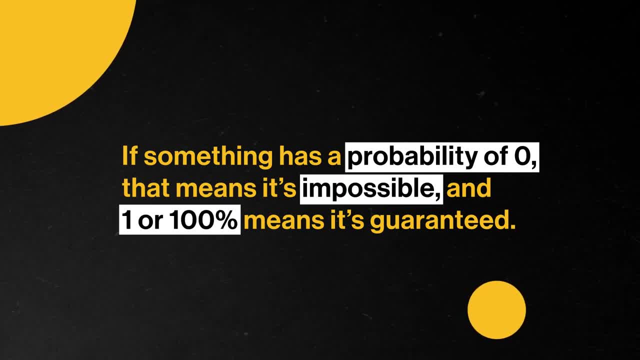 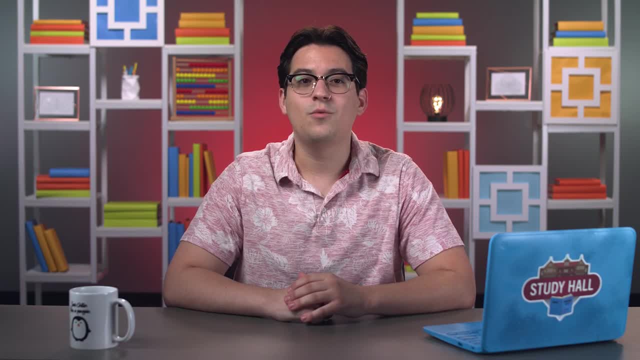 of 0,, that means it's 0.. That means it's impossible, And 1, or 100% means it's guaranteed. In this episode, we're going to start establishing rules that will help us find the probability of something happening when we combine events. Specifically, we'll learn how to calculate. 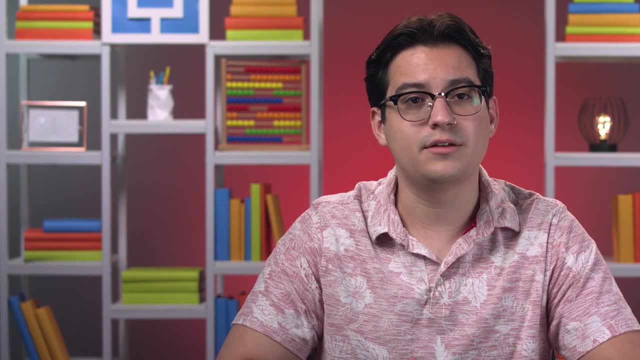 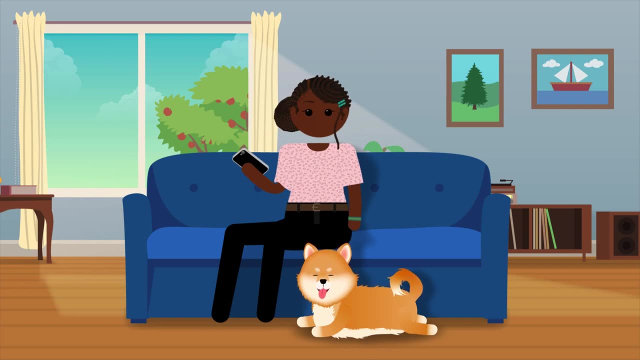 a probability when one event or another might happen and how we can use a table or a Venn diagram to figure it out. For people like Ebony, this could be helpful to make life-altering decisions like figuring out which store to shop at to avoid certain crowds. While scrolling on Twitter, Ebony stumbled upon a report. 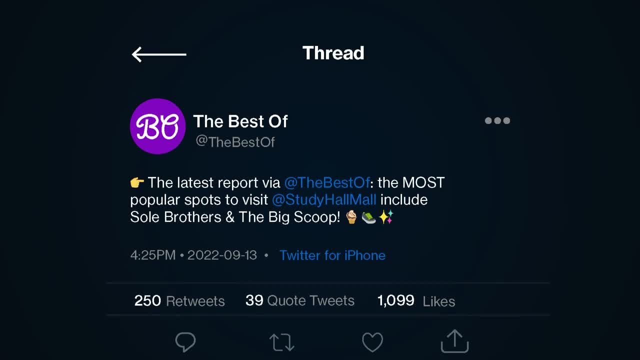 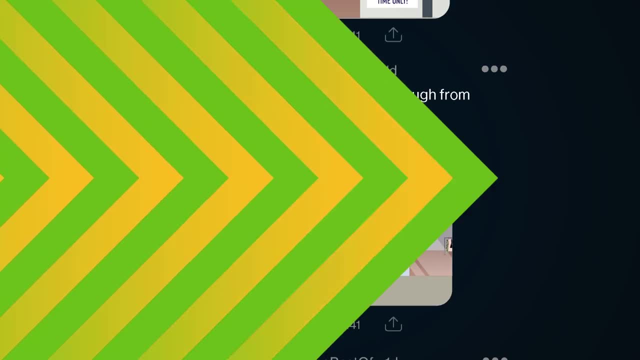 about the most visited stores at her local mall. On that list she saw her favorite shoe store that usually has the coolest sneakers, and that ice cream store everyone's been talking about with the best cookie dough ice cream. Now Ebony is willing to drop a fair amount of money at either store, but she's less. 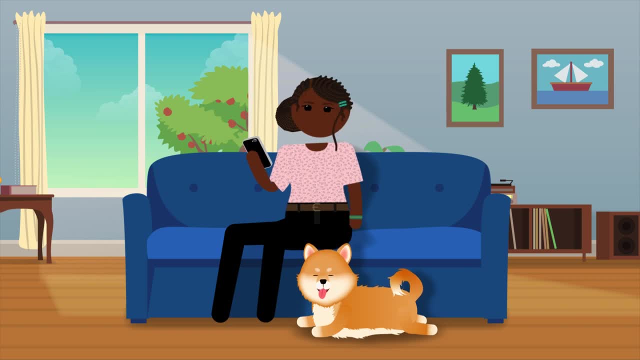 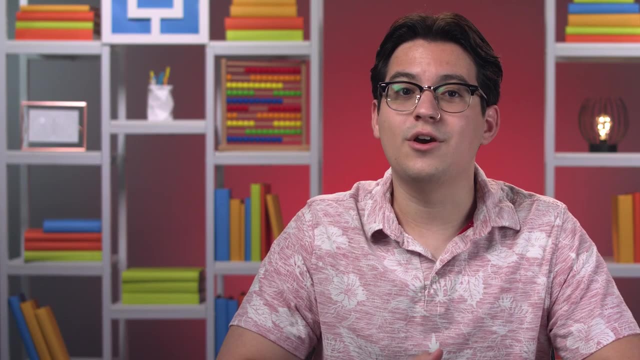 willing to deal with a crowd. So before she heads to the mall, she wants to know how likely it is that either store is too busy and crowded for her liking. And this is where things get… probable. Ebony needs to know the probability. other 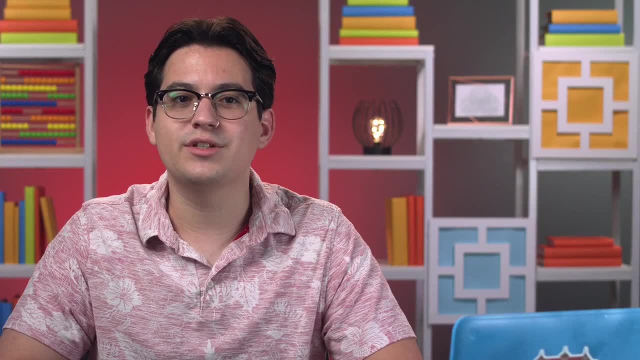 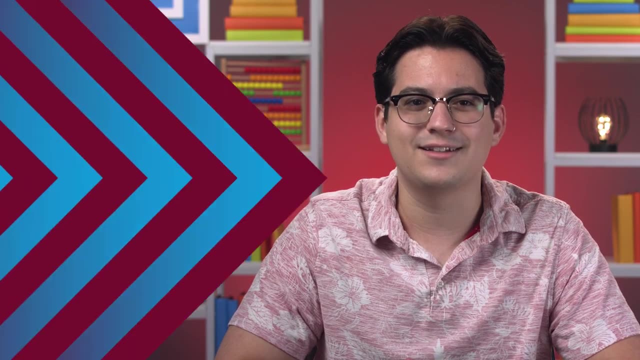 folks want to go to the same stores she does. On that trusted, well-respected and reliable report from Twitter, Ebony is going to figure out this math thing in the name of protecting her social anxiety. The report included a table with a week's worth of survey data from 1,000 people who went to the mall and 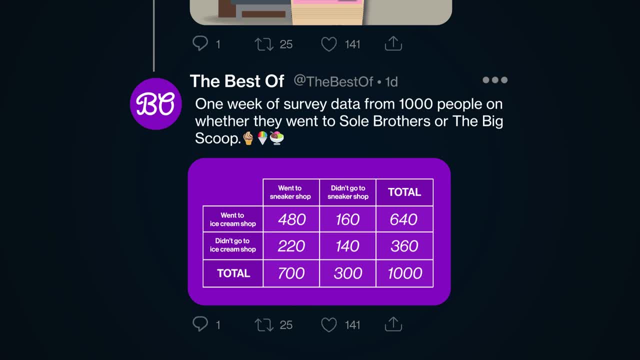 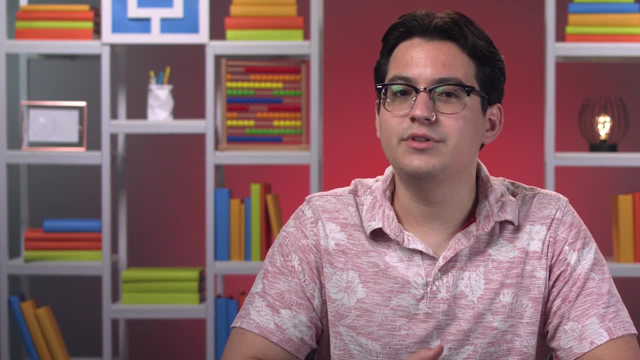 whether they visited the ice cream store, the shoe store or neither. Not sure why. the report conveniently only showed the data Ebony needed, but that's neither here nor there. The table tells her how many people did or didn't go to each store, but it doesn't. 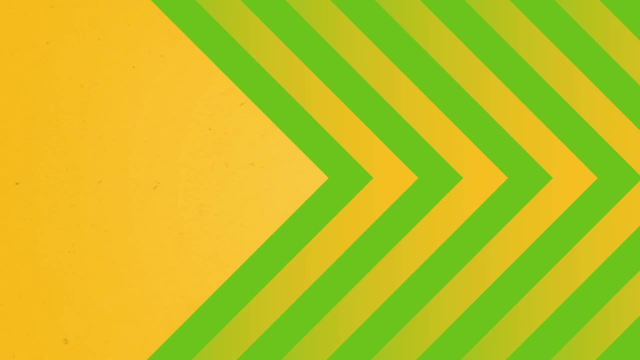 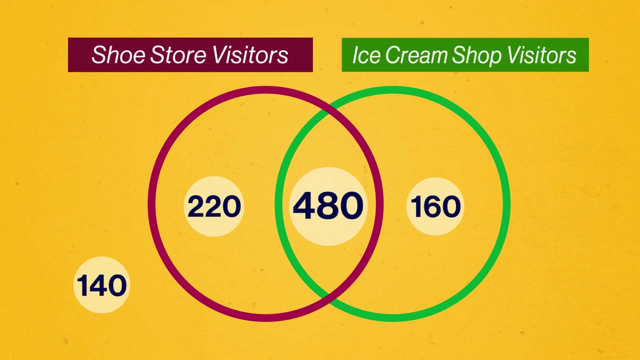 tell her how likely it is that people will be at both or neither store. Let's throw these numbers into a Venn diagram instead and think about it. We have one circle representing the shoe store and the other circle representing the ice cream store. Altogether Ebony figures that 700 people went to the shoe store at some. 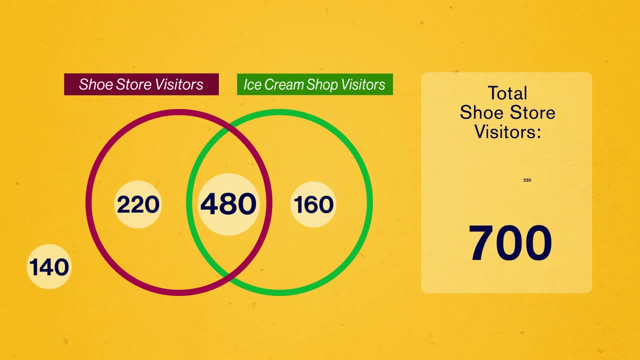 point out of the 1,000 folks sampled at the mall by adding the 220 people who only went to the shoe store and the 480 people who looked at shoes AND went to get ice cream. Then, to calculate the probability, someone from our sample went to the shoe store. we 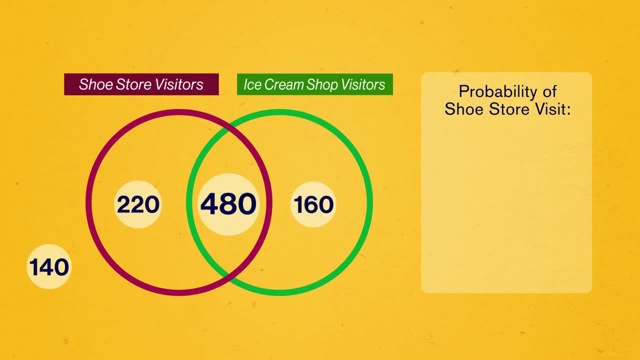 think of this as an empirical probability, because it's based on observations, and divide the number of people that went shoe shopping by the total number of observations. In math, we'd write that as the probability someone visits the shoe store equals 700 divided. 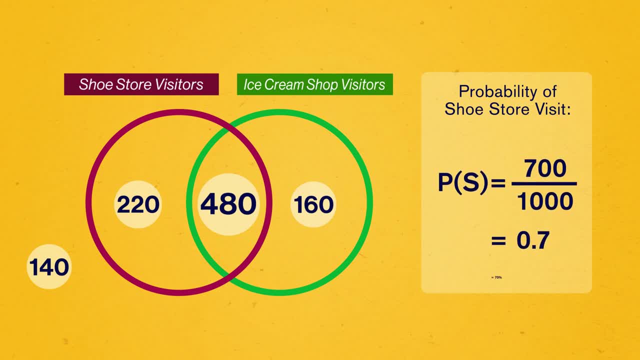 by 1,000, which equals 0.7, which can be converted to 70%. Assuming the 1,000 people surveyed are a good representation of everyone visiting the mall, that means we think there's a 70% chance a random person visiting the mall is going to go to the shoe store. So for Ebony, 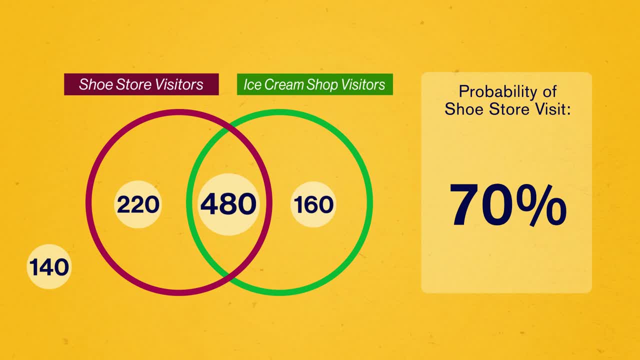 the shoe store is probably a no-go. We could look at this another way by figuring out the probability. someone didn't go to the shoe store. 160 people went to get ice cream and then 140 people were just elsewhere roaming the mall. So the probability of people not 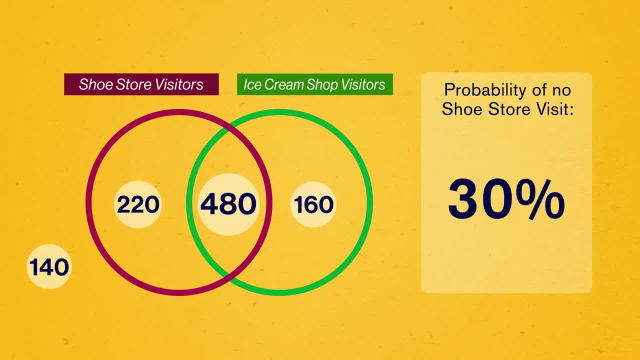 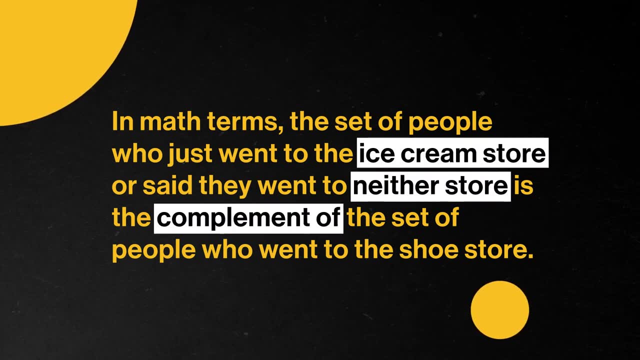 going to the shoe store is 300 divided by 1,000, or a 30% chance. In math terms, the set of people who just went to the ice cream store or said they went to neither store is the complement of the set of people who went to the shoe store. 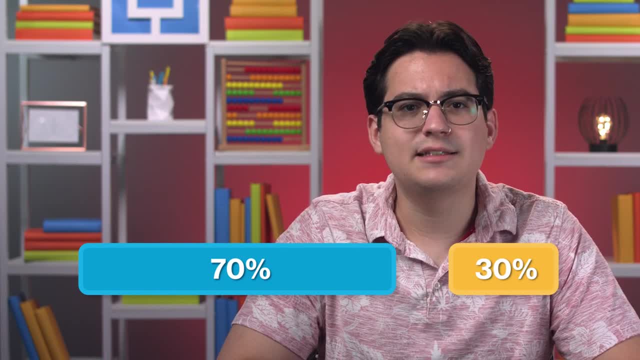 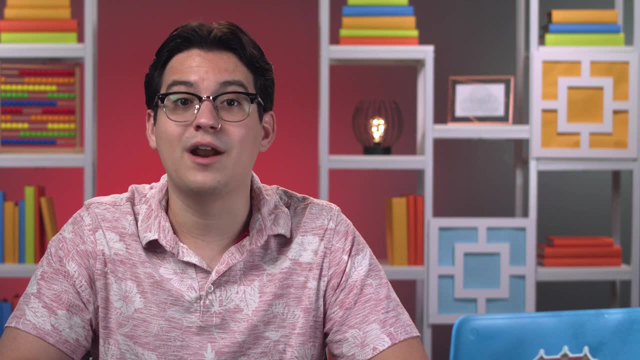 We talked about complements in our set operations episode and it makes sense that 70% and 30% add to 100% because a set and its complement should be equal. Ebony knows to avoid the sneaker store, but really she wants to know how likely someone. 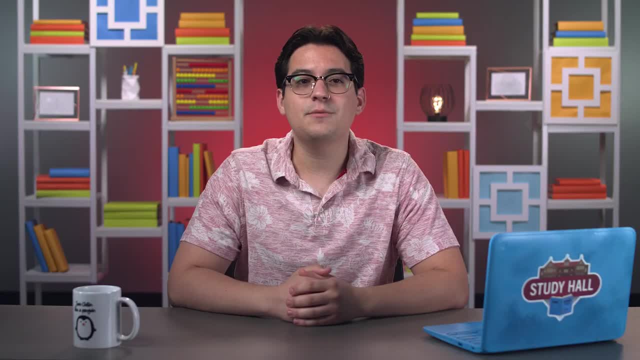 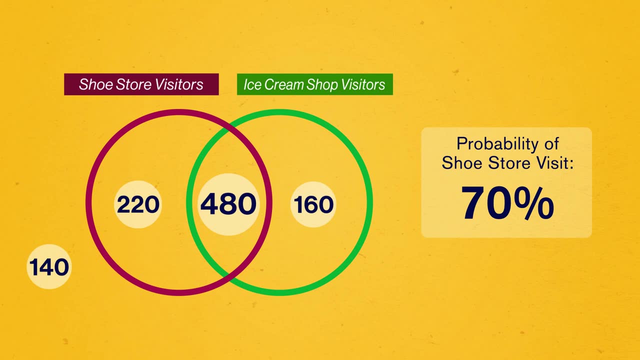 is to go to the sneaker store or the ice cream place. To really get the picture and accurate details, we need to consider our Venn diagram a bit more closely. We already know the probability of people going to the shoe store is 70% and by the 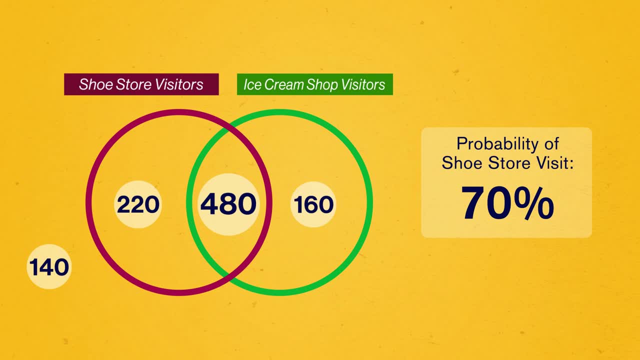 same method we just used. the probability of people going to the ice cream store is 64%. But to calculate both of those probabilities we had to consider the people who went to both stores. So to find the probability someone went to either store, we can't quite just add up. 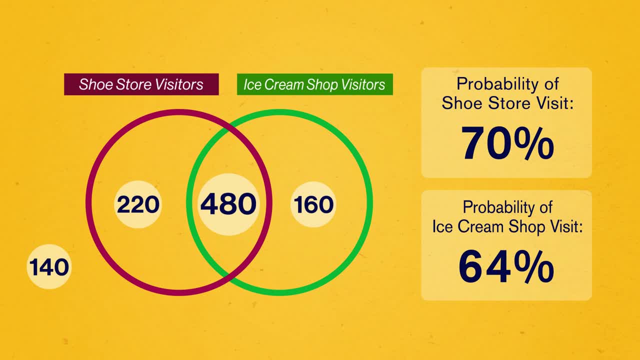 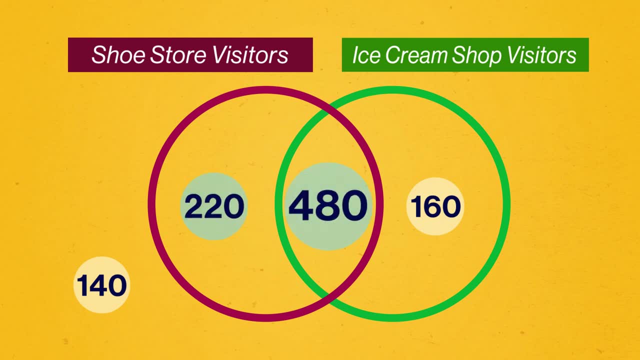 the probabilities because we'd be factoring in the people who went to both stores twice. Our Venn diagram is useful for visualizing here. To calculate the probability of people going to the shoe store, we added everything in the first circle. Then, to calculate the probability of people going to the ice cream store, we 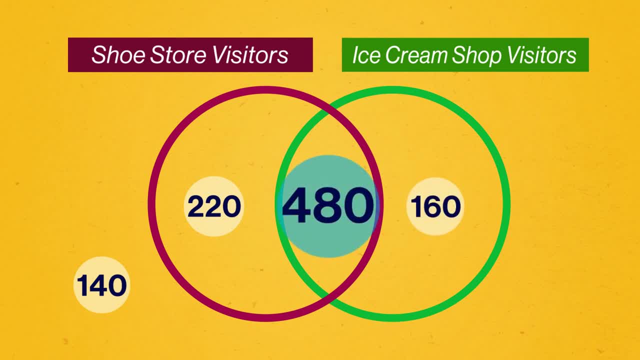 added everything in the second circle, So we counted the part where the circles overlap twice. Fortunately, at some point in our rich mathematical history, mathematicians figured out how to clear this double counting up. We just… figure out how to count the overlapping part once, Sweet. 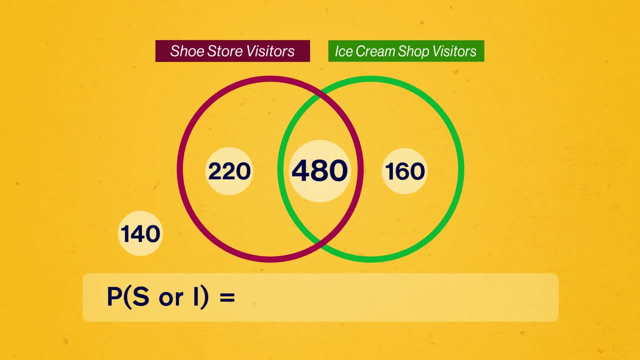 So the probability of going to the shoe store OR going to the ice cream shop is the probability of going to the shoe store plus the probability of going to the ice cream store, minus the probability of going to both spots. Actually, what we've done here is recreate a formula that we can use any time we want. 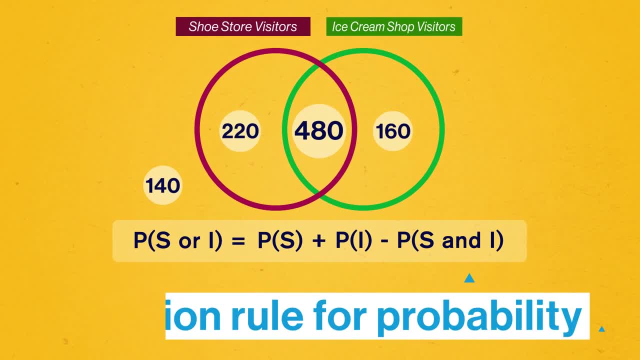 to find the probability of one event OR another happening. We call this the addition rule for probability. If we label our shoe circle S and our ice cream circle R, we get the probability of going to the ice cream store plus the probability of going to the ice cream store, minus the 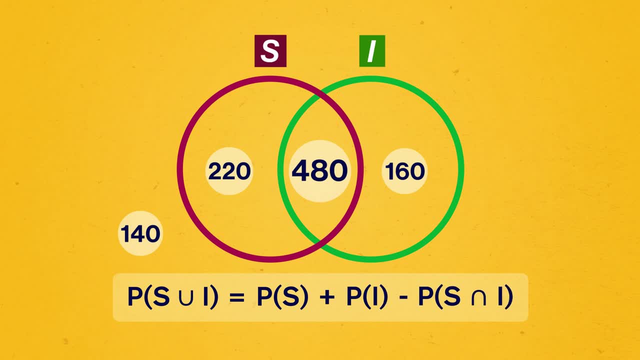 probability of going to the shoe circle I. then we can write the addition rule using set notation. You can see we subtract out the middle overlapping area of the Venn diagram, so we only consider the part where the sets overlap. once Working through that formula, we find that there's an 86% probability that Ebony will. 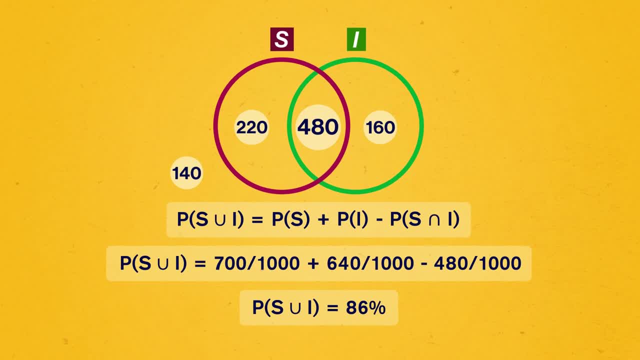 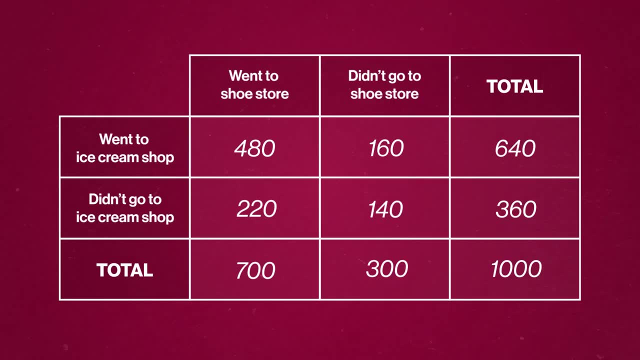 have to run into somebody at either store, no matter what Them's the breaks. Making a Venn diagram is really helpful when we're trying to visualize complicated sets, But we could have also done these calculations using the original table from the report. 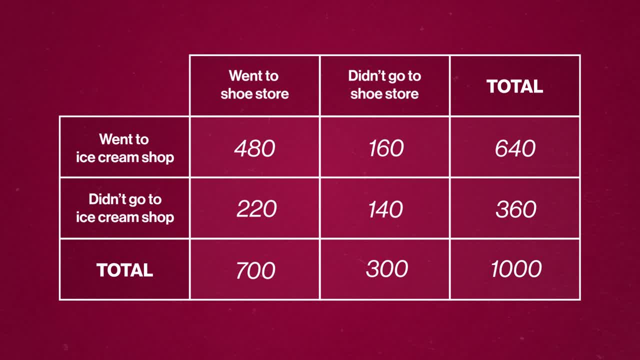 If we divide everything in the table by the number of sets, then we get the probability of going to the ice cream store plus the probability of going to the ice cream store, minus the number of sets, plus the number of people who were surveyed- the 1000, then we would.